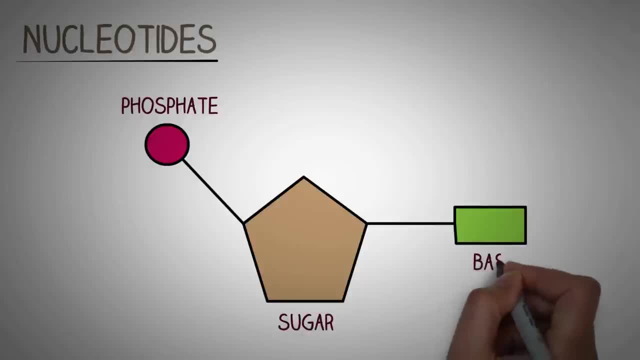 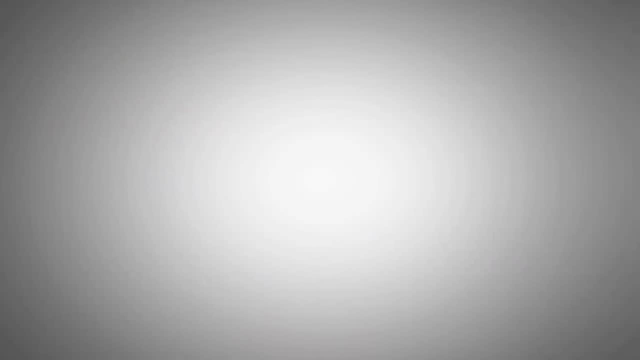 the sugar and the nitrogenous base, and these groups are attached to one another by bonds which we will discuss later. To understand the complete structure of a nucleotide, let's try to understand the structure of these groups one by one. So the first is the sugar, The 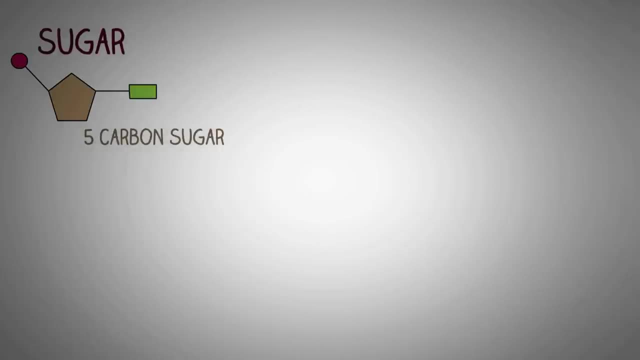 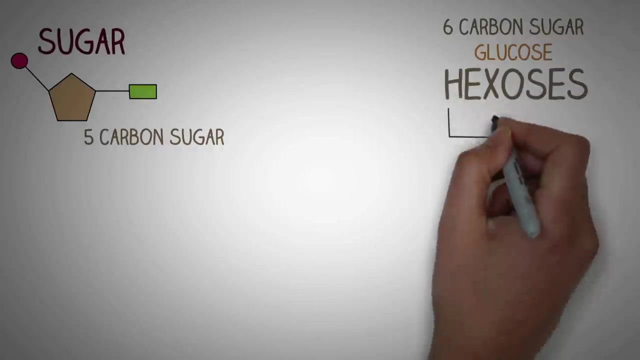 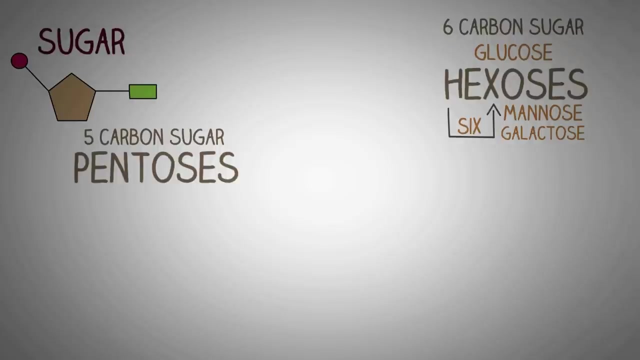 sugar present inside the nucleic acids are five carbon sugars. Now most of you know the different types of pentoses in our body, but the two important types of pentoses that are present inside the nucleic acids are pentoses and pentoses are pentoses. So pentoses are. 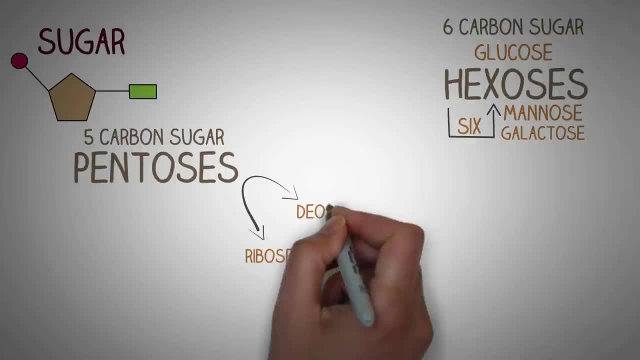 pentoses and pentoses are pentoses and pentoses are pentoses and pentoses are pentoses. So if we compare this structure with the chemical structure of the ribose and deoxyribose on the right, we can see the structure clearly. We have carbon atoms on each of these corners. 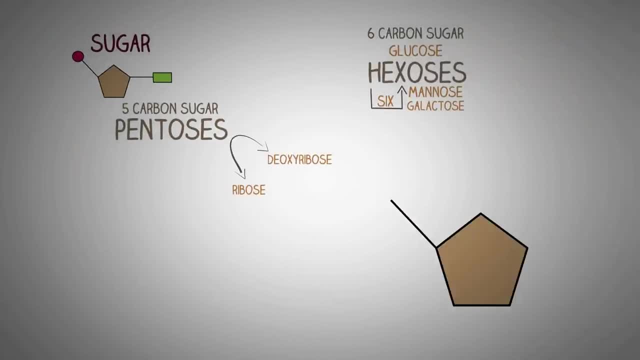 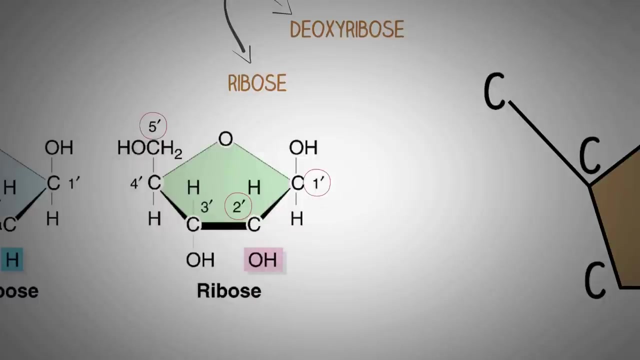 Note that the last carbon atom is located outside the ring. We have an oxygen atom at the center top most position. We can also see in this chemical structure that the interactions that the carbon atoms are named from 1 to 5 in a clockwise direction, so the 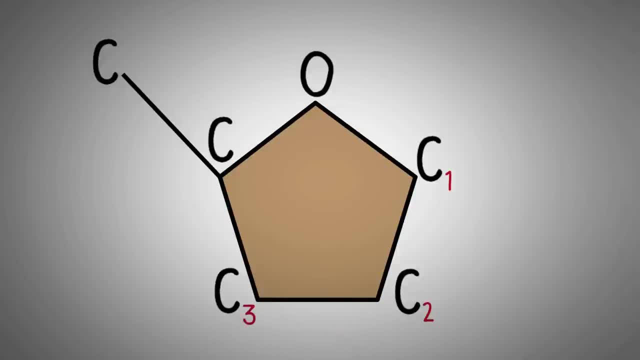 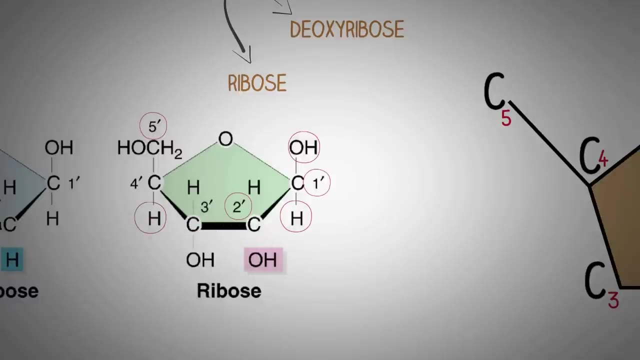 carbon atom next right to the oxygen is called c1, so c2, c3, c4 and c5. c5 is located outside the ring. you can also see in this chemical structure we have different type of functional groups attached to these carbon atoms, like the hydroxyl group and the hydrogen atom, the most important of these functional 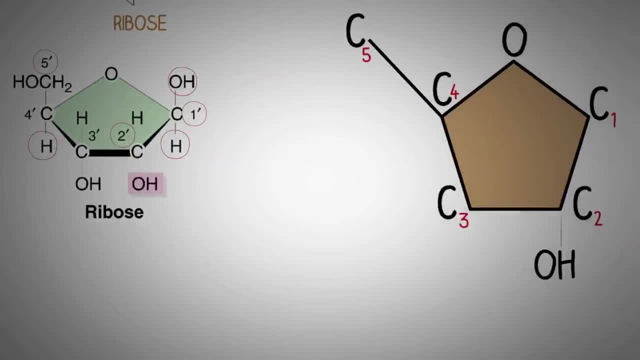 groups which determine whether the sugar is ribose or deoxyribose are present at the carbon number two and the carbon number three. in the sugar ribose we have a hydroxyl group that is attached to the carbon number two. this is the chemical structure of ribose. now, if you compare this structure with the structure of 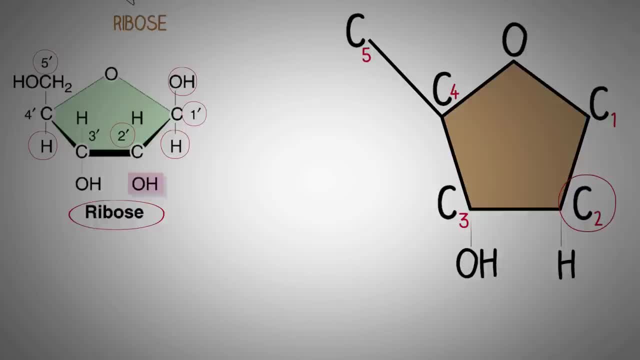 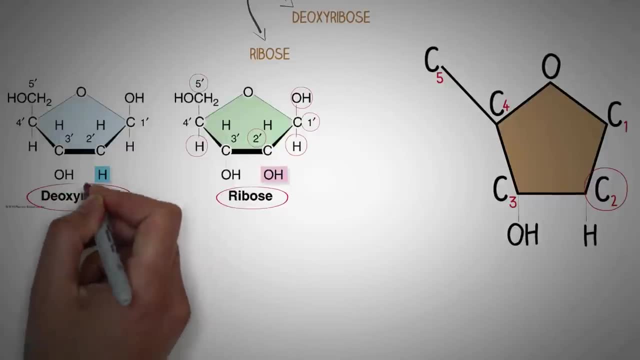 deoxyribose. the only major difference is that carbon number two, that the carbon number two contains only a hydrogen atom and not the hydroxyl group. so the resultant sugar is called a deoxyribose. here you can see the carbon number two in deoxyribose contains only a hydrogen. 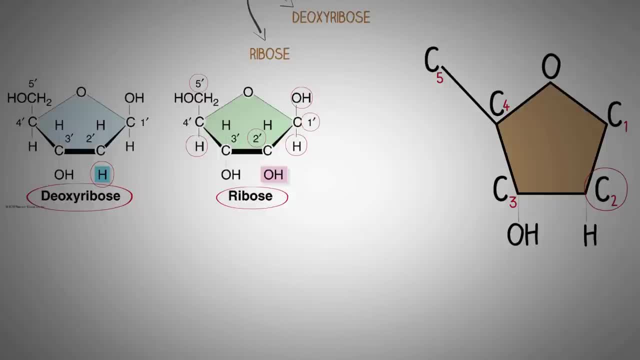 atom, whereas in ribose, the carbon number two contains a hydroxyl group. you can also tell this by the difference in their names, that the deoxyribose has a prefix called as deoxy, which means removal of oxygen, the resultant sugar. the deoxyribose is more stable as compared to ribose because of one less. 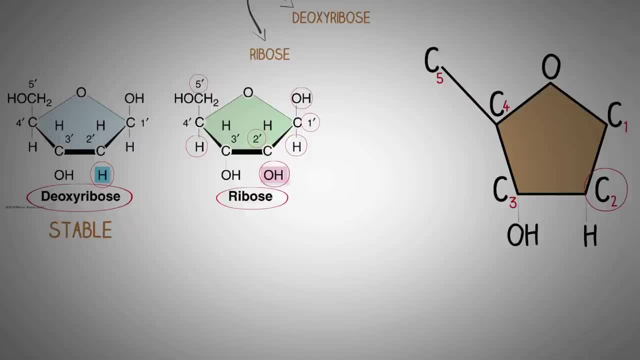 functional group: the deoxyribose is present in DNA and ribose is present in RNA. you can also remember this by the starting of the DNA, which starts with D, so the deoxyribose, and the RNA, which starts with R, so the sugar is the ribose. 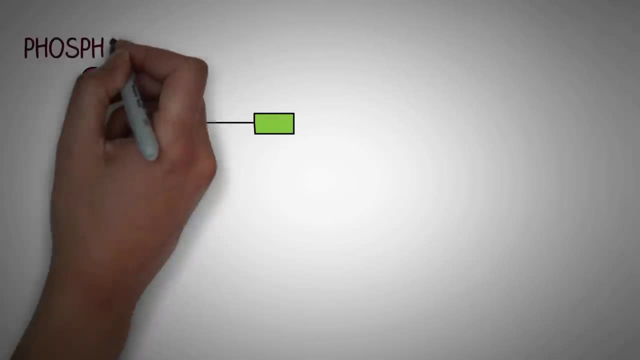 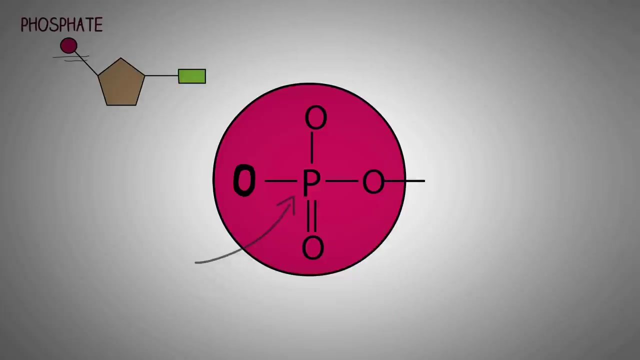 the next important group to study in a structure of nucleotide is the phosphate group, which is this entity right here? the phosphate group consists of a phosphorus atom in the center to which four oxygen atoms are attached which are negatively charged. the phosphate group is the same phosphate group which is present in the 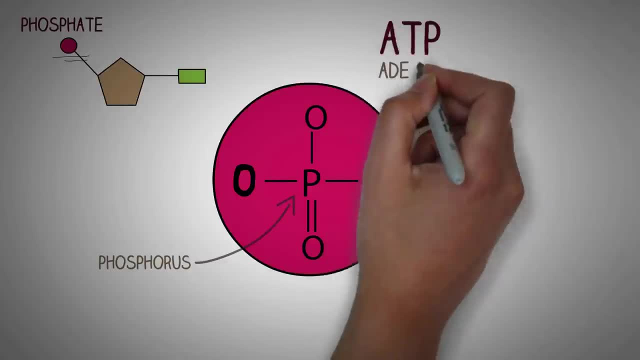 adenosine triphosphate, the energy carrying molecule of the body. however, in ATP we have three molecules of phosphate which are attached to one another by high-energy phosphodiester bonds. the phosphate group is a polar molecule due to the presence of highly ionized oxygen atoms which impart negative charge to. 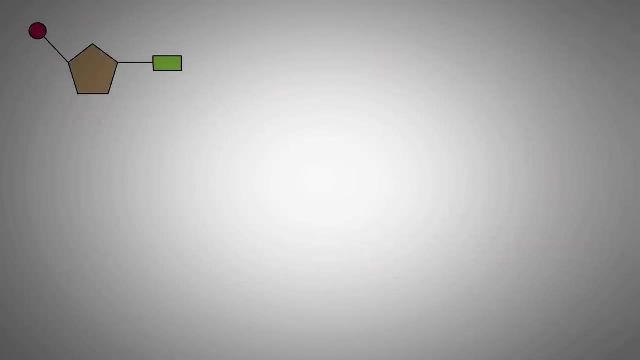 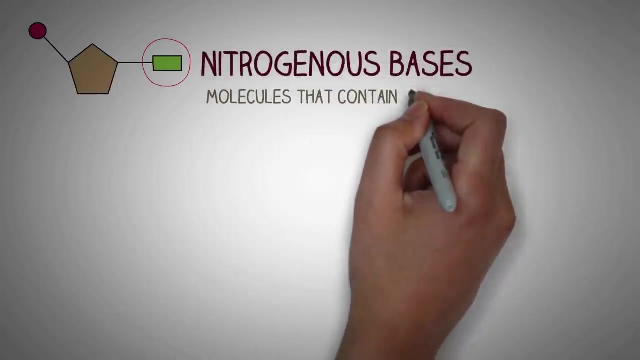 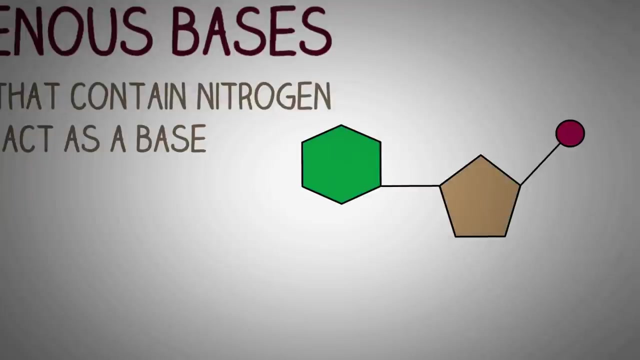 the phosphate group. now the third important structure present in the structure of a nucleotide is the nitrogenous base. nitrogenous bases are basically molecules that contain nitrogen in varying amounts and they act as a base. most of you know that the human body contains organic chemicals which have carbon, hydrogen and oxygen in varying amounts in nitrogenous bases. 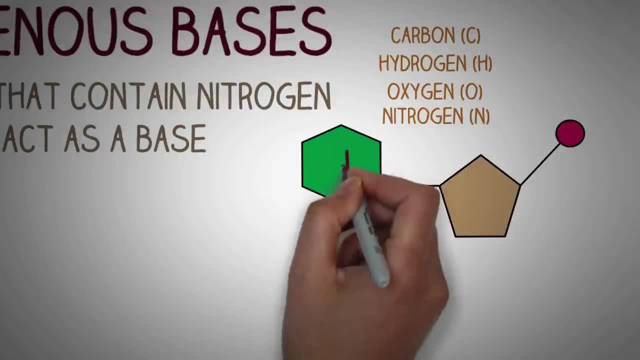 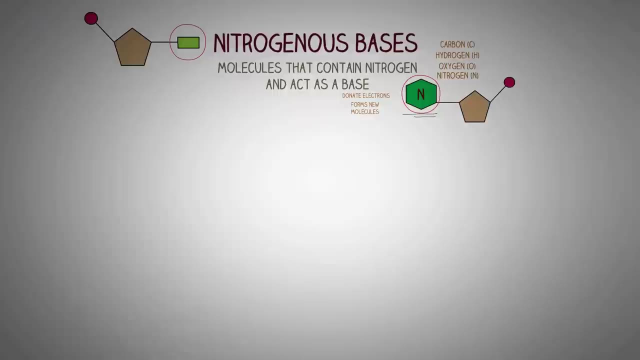 nitrogen combines with all of these atoms to form ring-like structures. these molecules are called bases, since they can donate electrons to other molecules and form new molecules. in this process, the nitrogen combines with all of these other atoms to form ring structures. now we can have two different types of ring. 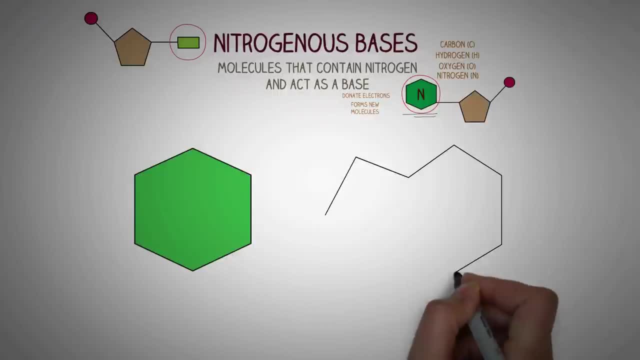 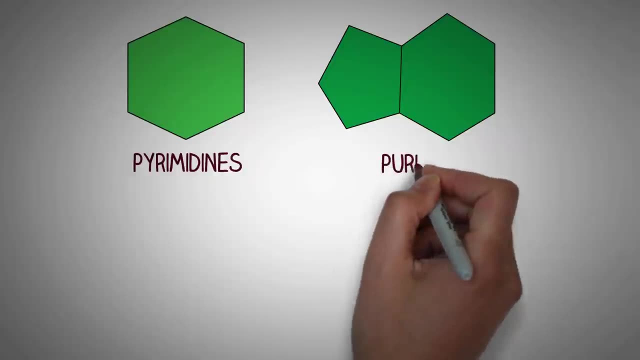 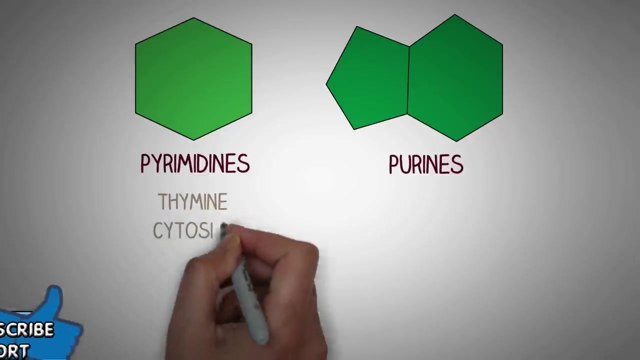 structures: one where there are single rings and second where there are double rings. the single rings are called pyrimodines and the double rings are called purines. we have three different types of pyrimidines: the thymine, cytosine and the uracil, and we have two different types of purines called adenine. 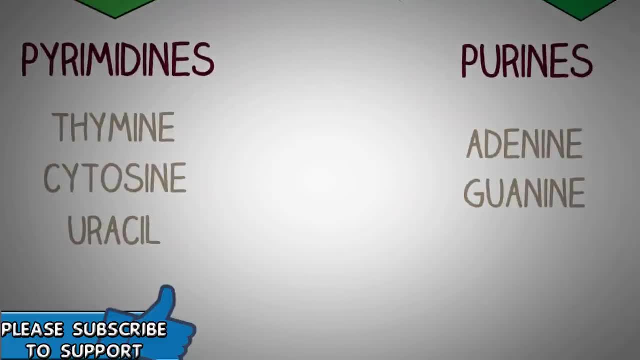 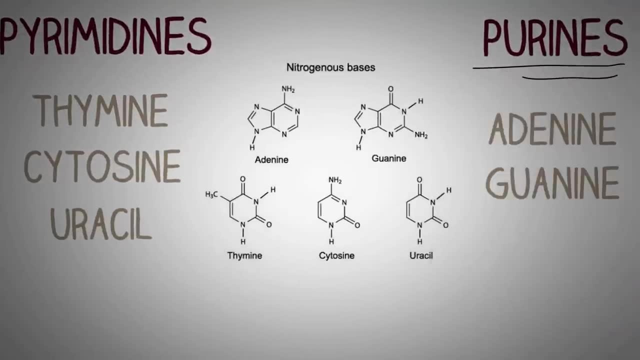 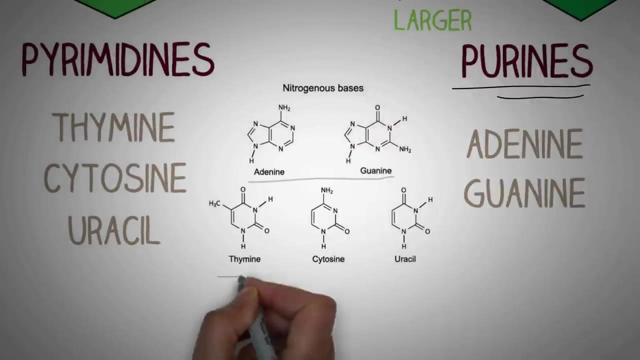 or and guanine. In the center you can see the chemical structure of each of these bases. As you can see, the purines which are double ringed structures: adenine and guanine. Due to the presence of double rings, these purines are larger as compared to the pyrimidines. 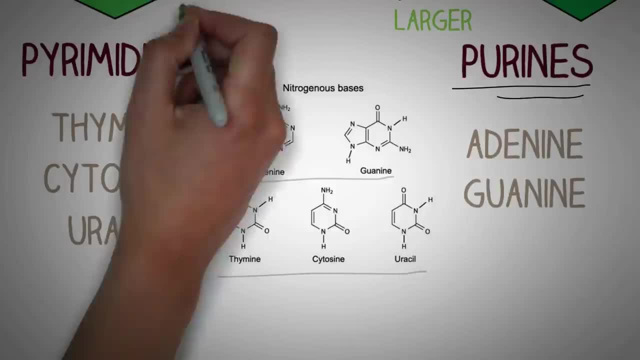 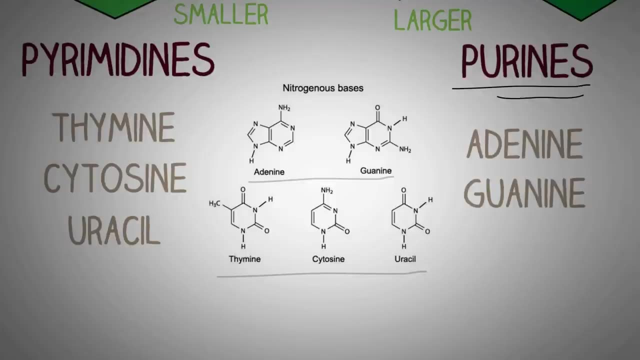 The thymine, cytosine and uracil all are single ringed structures and they are smaller as compared to the purines. The difference in the size of these bases is very important, as it helps to pair these bases in the structure of DNA properly, which we will study later. 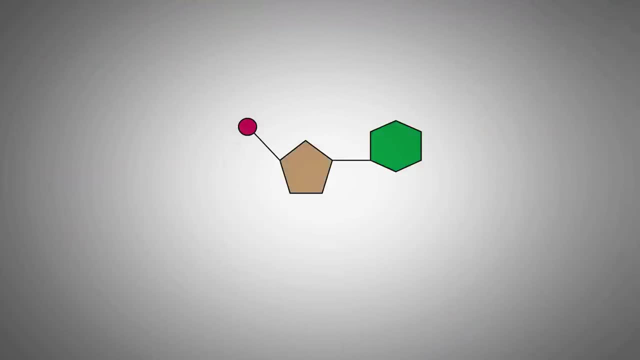 So now you know the individual structures which are present in a single nucleotide. Next we will look at how these individual structures bond to each other to form a single nucleotide, and then we will look at how many nucleotides bind to each other to form a chain. 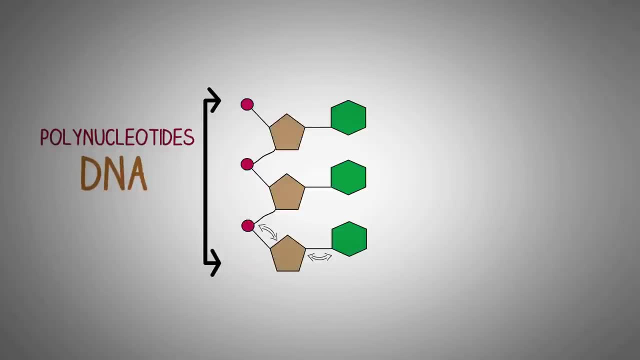 of nucleotides, which is called a polynucleotide, which can be either DNA or the RNA. So if we take a sugar and name just the important carbon here, which will be the carbon number 1 and the carbon number 5, and of course you can. 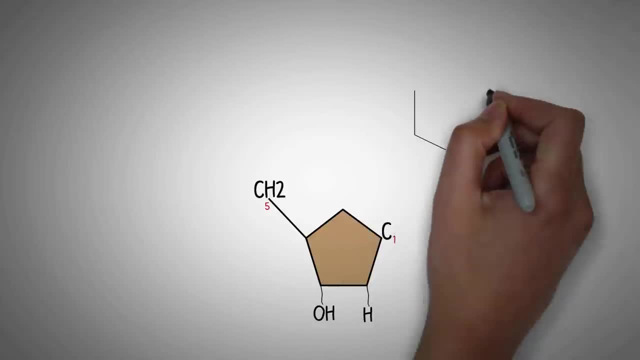 see that at the carbon number 2 there is only a single hydrogen atom. so this sugar will be a deoxyribose. Now to pair this deoxyribose sugar with this pyrimidine ring, the bond formed will be between the N1 of the pyrimidine ring and the C1 of the sugar. 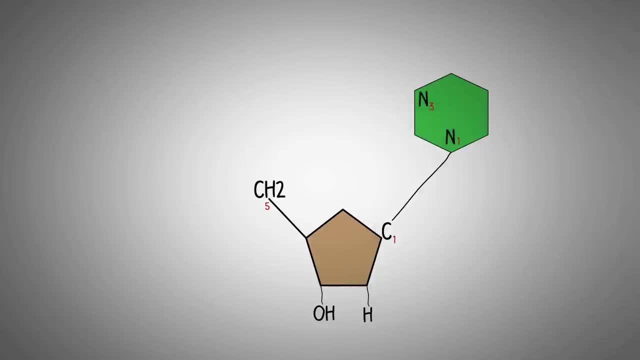 If you want to go into the details about how these nitrogens are named, you can check the link in the description below for the IUPSC nomenclature of the aromatic compounds. So let's get started Now. this bond will be an example of a glycosidic bond, which is a covalent bond which links. 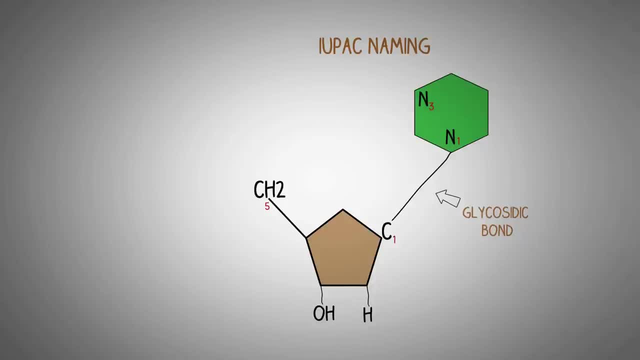 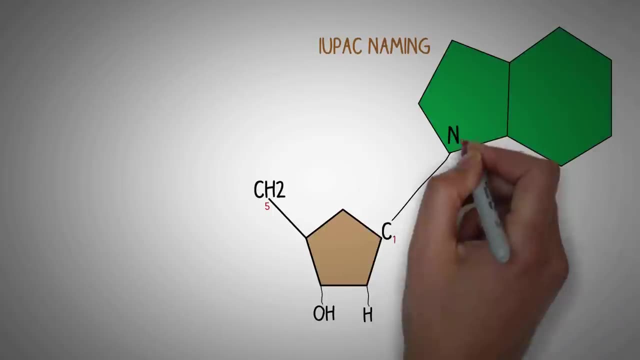 carbohydrates with other structures. Now if we have to pair a purine ring at a similar position, the bond formed will be between the N9 of the purine ring. Now next let's attach the phosphate. The phosphate group attaches with the carbon number 5 of the sugar and the bond formed. 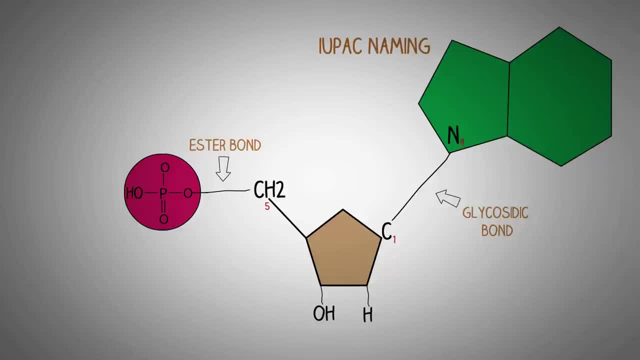 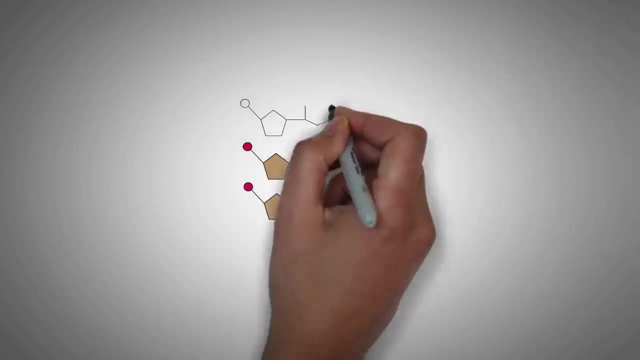 is the example of ester bond, Which is also a strong covalent bond. So now you know how the three structures in a single nucleotide bind to each other to form one nucleotide. Next, if we look at how many nucleotides bind to each other to form a chain of nucleotides, 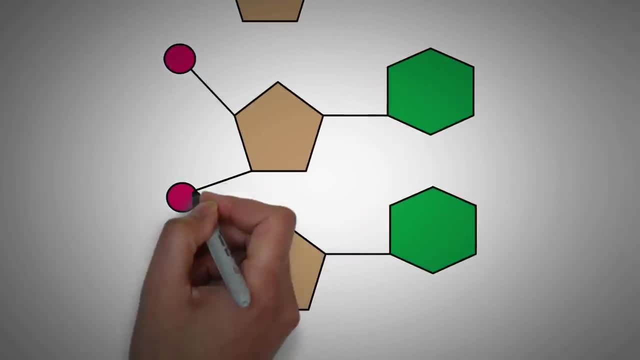 called polynucleotides. So you can see. basically, what happens is that the phosphate group that attaches to the carbon number 5 of the sugar below also forms a bond with the carbon number 3 of the sugar above, And this pattern is repeated again and again. 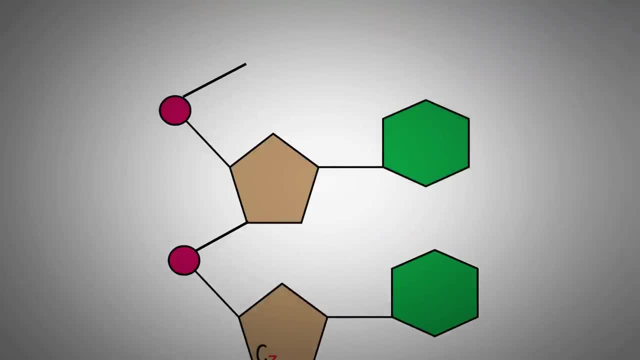 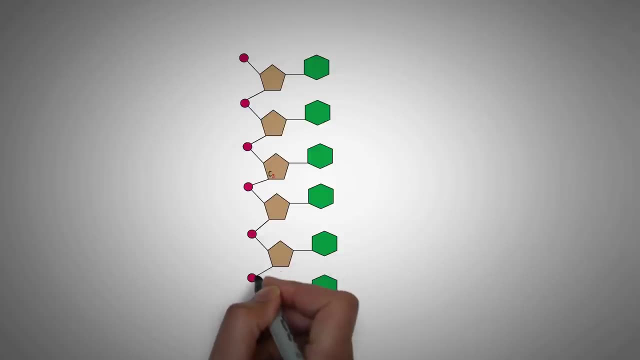 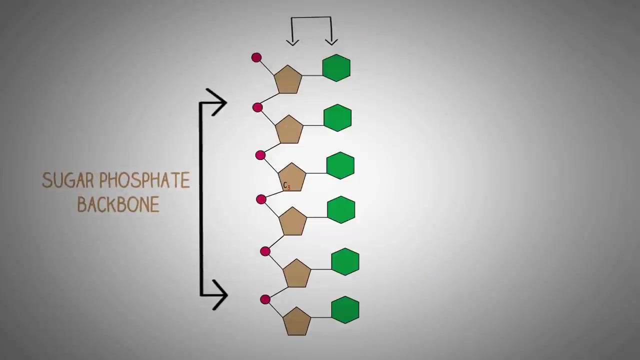 So you can see that the phosphate groups form bonds both above and below the chain of these nucleotides. So, as a result, a long chain of nucleotides is formed which consists of the graphungen of a sugar phosphate backbone, and in the center we have all these nitrogenous bases which 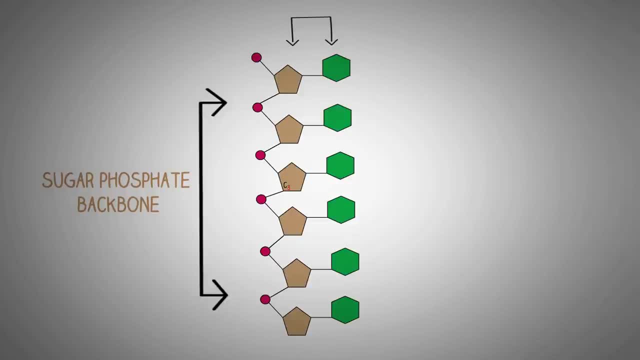 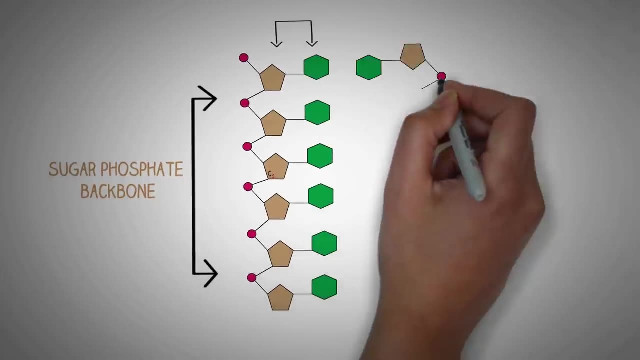 project from the sugar phosphate backbone. Now this can be an example of RNA. Yeah, present in this example will be a ribose sugar. but if we take a similar strand of polynucleotide and run it in opposite direction and this strand binds with the, 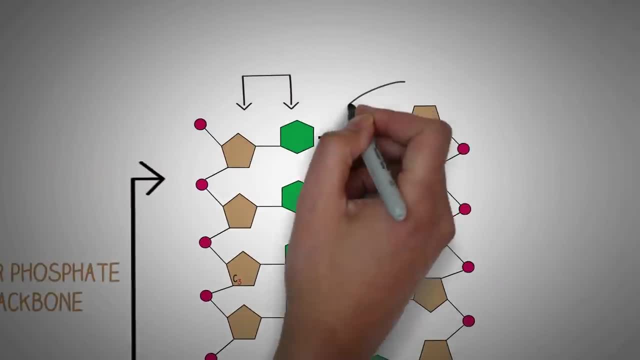 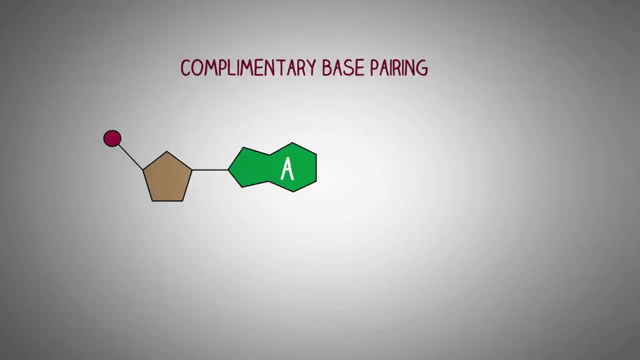 original strand through hydrogen bonds. now here comes a role of complementary base pairing. now, what complementary base pairing says that only adenine forms a hydrogen bond with thymine and only guanine forms a hydrogen bond with cytosine. now, this is a universal rule that is applied in the structure of 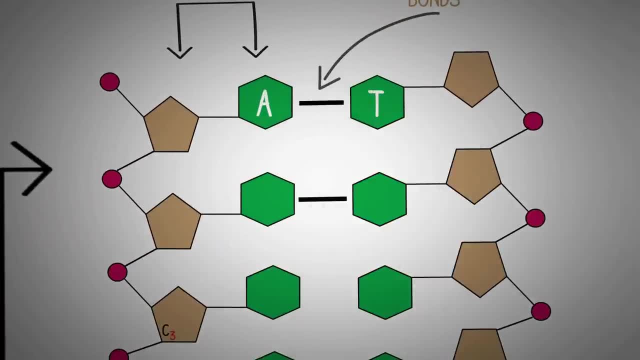 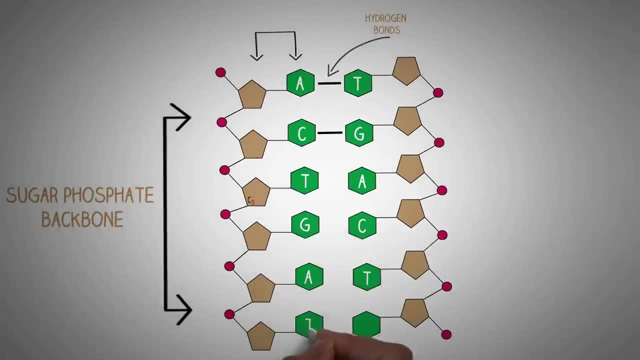 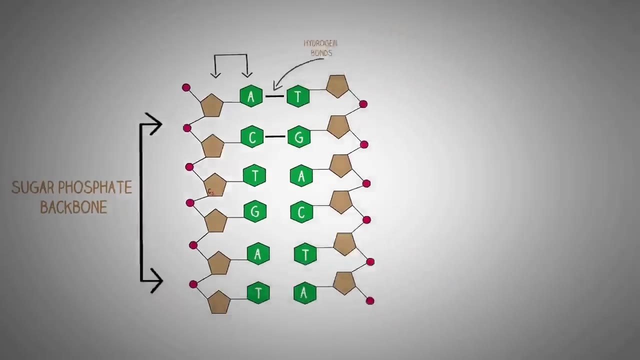 a DNA. so here you can see, adenine forms a hydrogen bond with thymine and similarly, thymine form hydrogen bond with only adenine. in a similar case, guanine forms a hydrogen bond with cytosine and vice versa. now, this, This is the basic structure of DNA, and you can compare this with the step ladder structure. 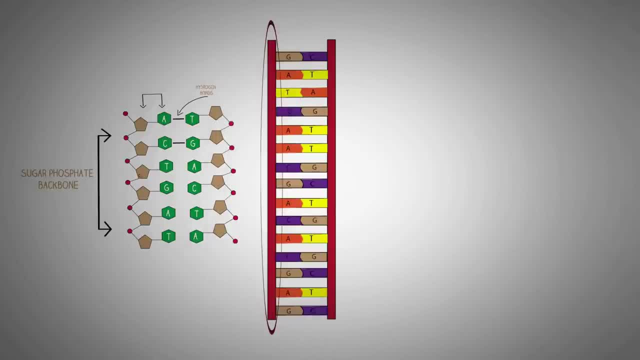 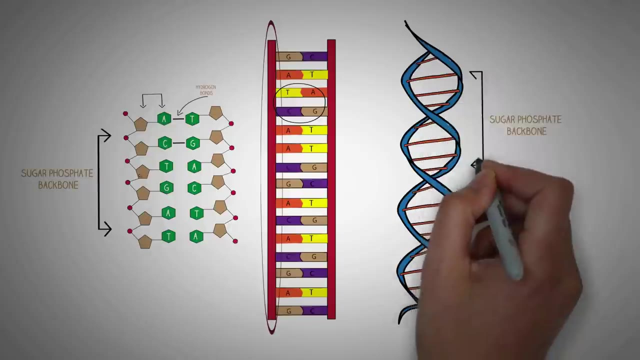 of the DNA. You can see that the supports of the ladder in the red are basically representing the sugar phosphate backbone, and the rungs of the ladder represent the nitrogenous bases that are forming hydrogen bonds with each other. Now, of course, the original structure of DNA is that of a double helix, so you can compare.